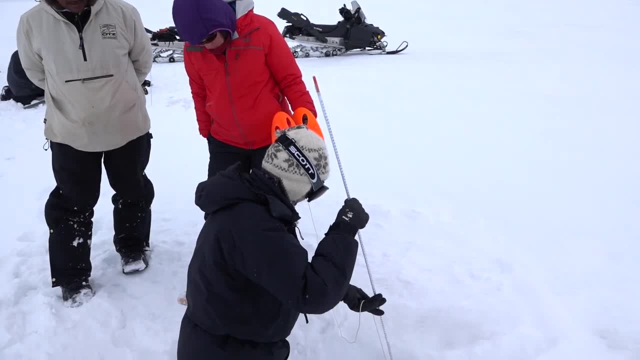 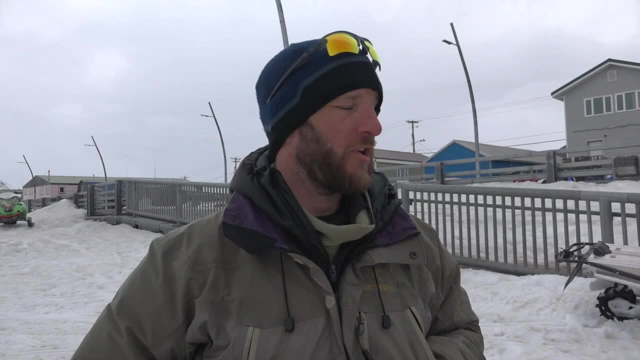 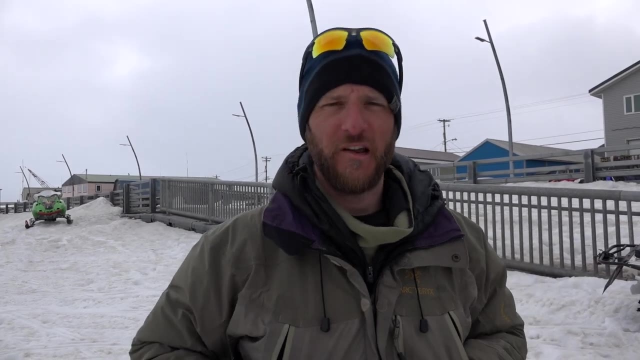 out on the sea ice with local elders and western scientists to look at seal habitat and any evidence of impacts due to warming climate conditions. We're getting ready to head out in a big convoy of snow machines out to an abandoned seal lair that we found out near one of Cyrus' hunting locations near Susolik. We're going. 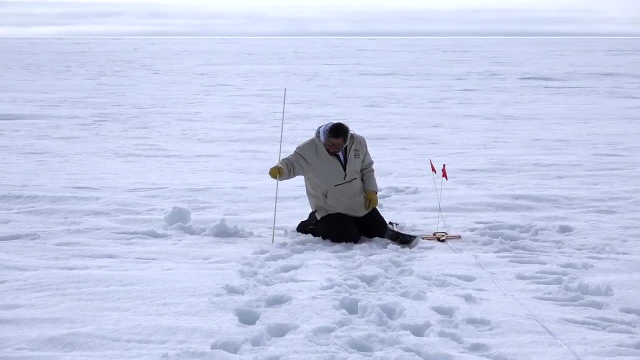 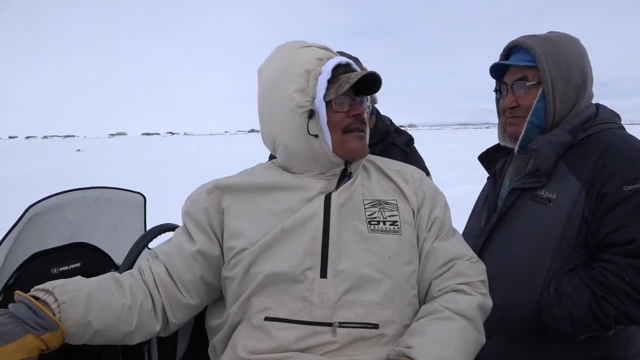 to go out there. We're going to go out there and take some measurements of the ice and snow and see what kind of ice and snow the seals choose to build their lairs in. We've got three of our advisory council members, three of the local experts on seals and sea ice here: Bobby Cyrus and 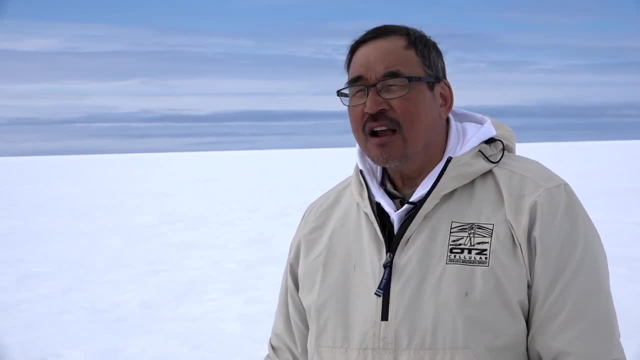 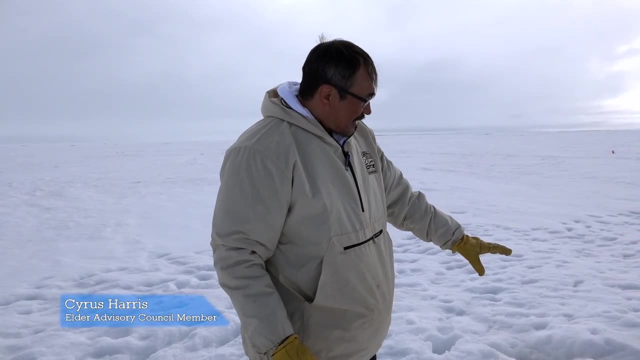 John are going to come out with us, so really looking forward to a good day of learning about ice and snow and seals. I'm saying this is a den that did get caved in with the warmer weather that we've been having here And it appears, with that little shelving in there, that the ice and snow are still. 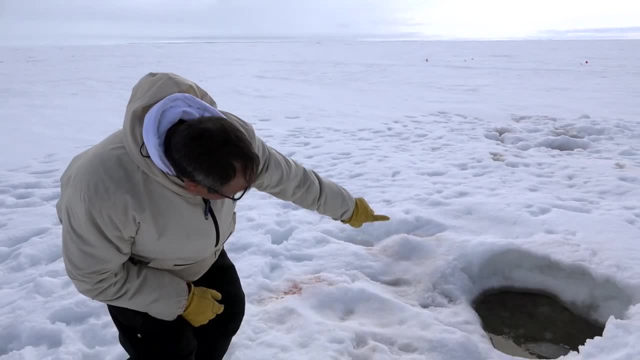 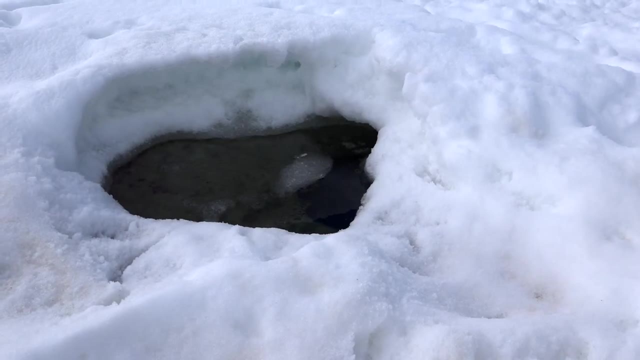 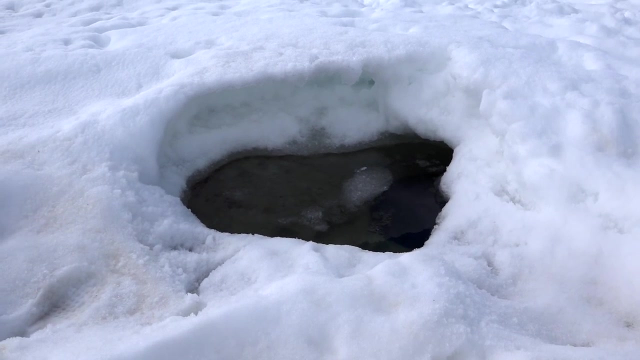 there, it appears that the pup might be protected from predators such as a raven. What creates these little snow banks is little ice piles in the ideal place for them to be making dens, but there's more ice piles within the area which they use for breathing holes and possibly dennings like this here. 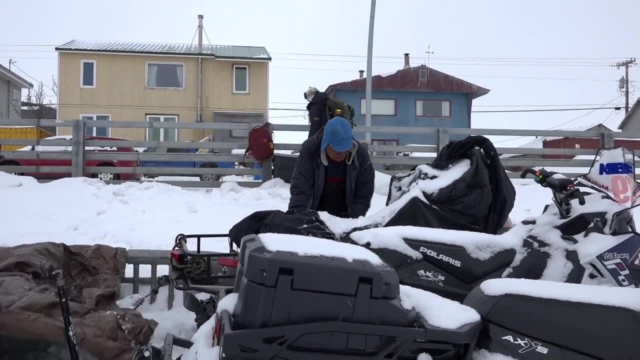 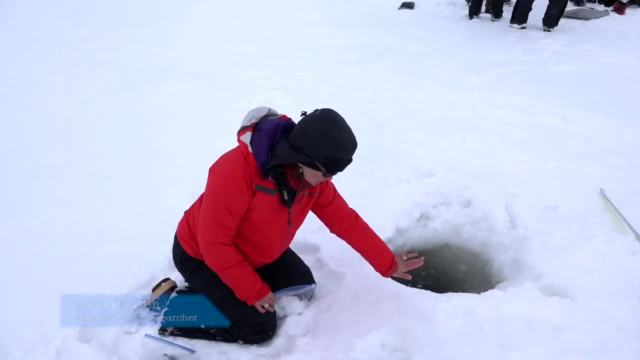 We are packing the gear and the sleds, going out with John and Cyrus looking at ringed seal habitat. You can see that the seal had hauled out and it was actually sort of iced over just slightly because of their warm body melting the snow around it. 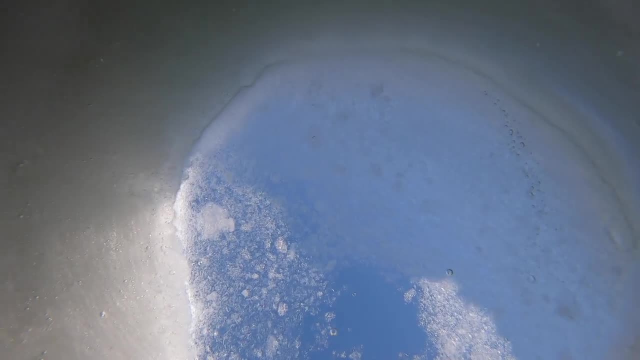 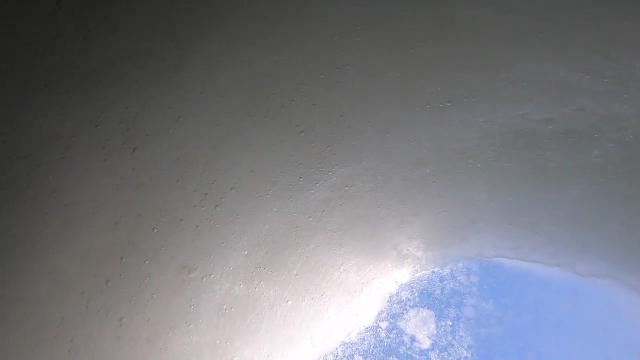 This particular breathing hole has a bit of a slope to it. You can tell that the seal usually entered from this direction out. this way There's some kind of sloping to the walls. Even just for indicators of melt. there can be interesting pitting. 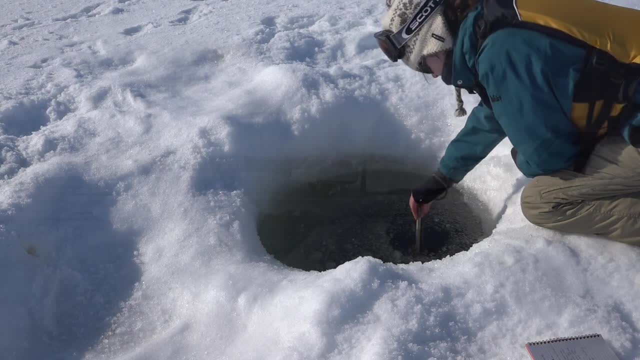 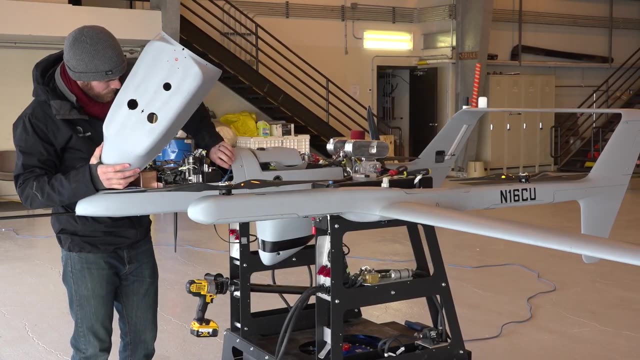 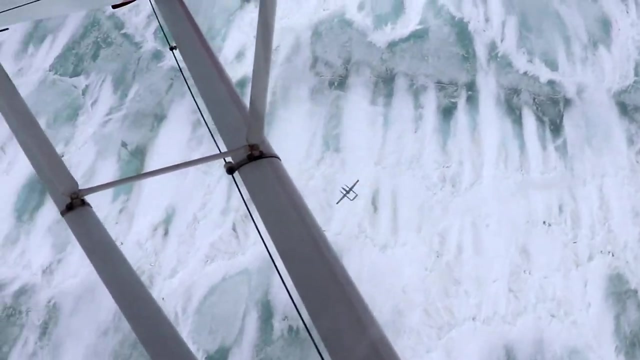 on the seal, The surface of the ice, from below. Our aerial surveys were done by the use of scientific instrumentation called payloads in the head of large fixed wing drones that flew over areas of Kotzebue Sound, The thermal visible payload, which is what we use to survey for seal habitat. 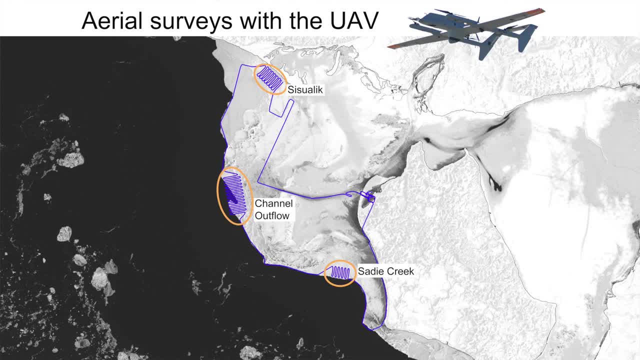 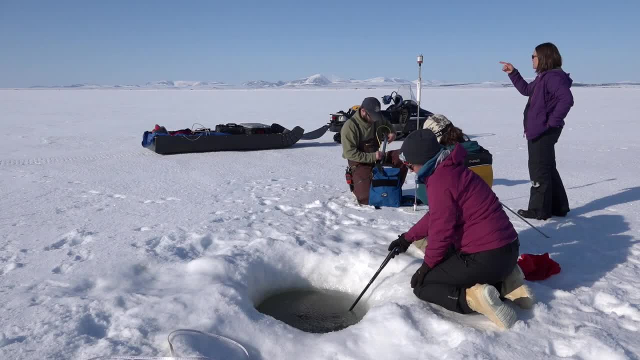 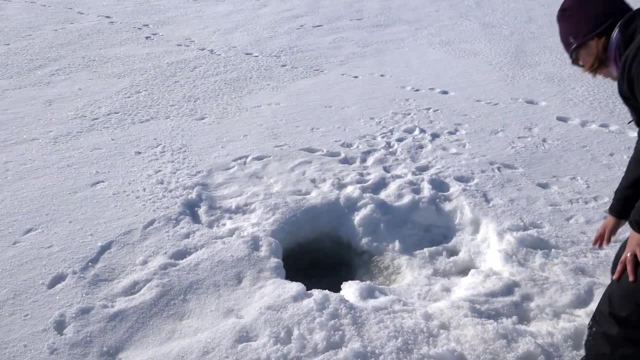 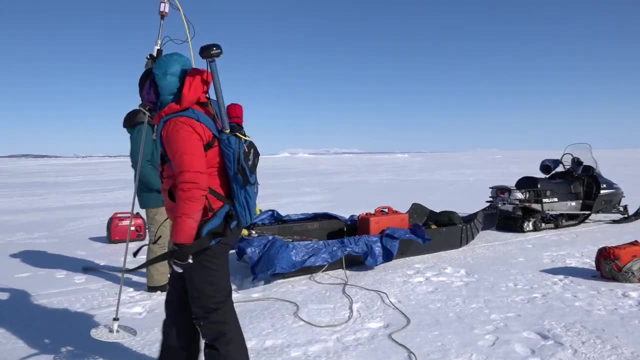 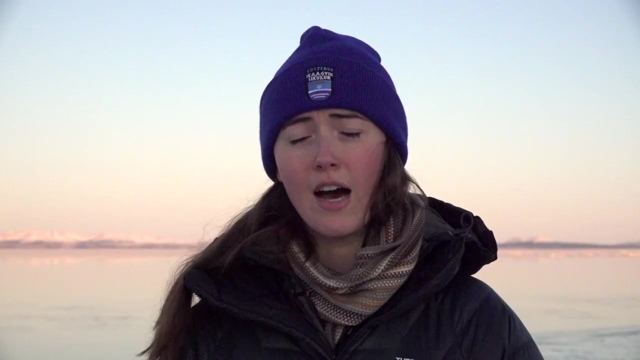 that we've confirmed on the ground have seals and have seal structures, and we can also fly over locations where we've done topography surveys and surveys for snow depth, so we'll have data on what that ice surface is like to pair with our observations of seals from that location. 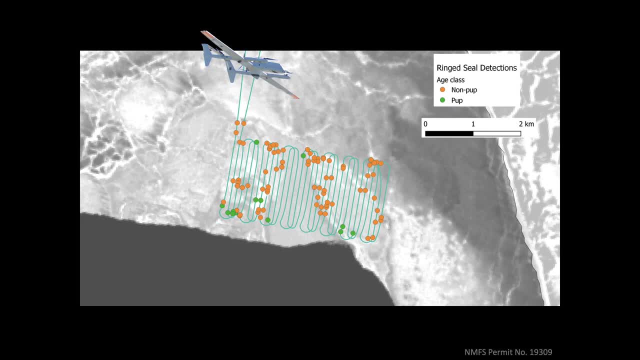 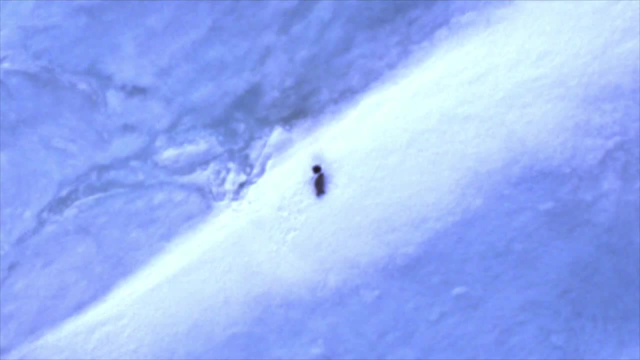 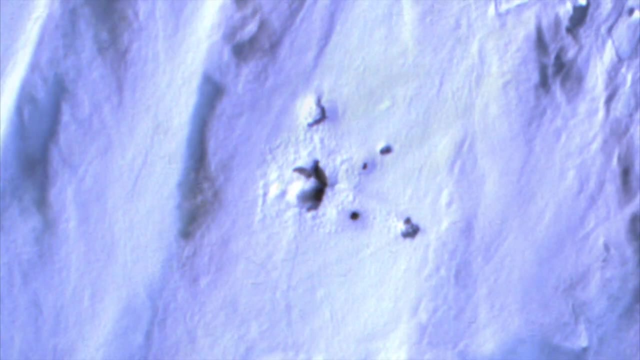 I'll be looking at all the different locations. I'll be looking at all the different locations where we saw ring seals on the sea ice in the drone imagery and trying to see whether there's a systematic difference in where we saw seals and where we didn't, so we can look at what habitat features they're selecting for, such as 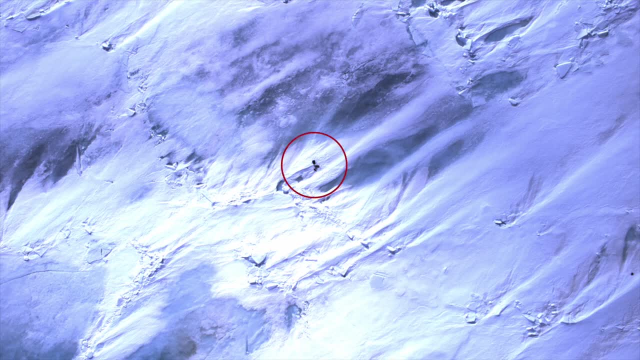 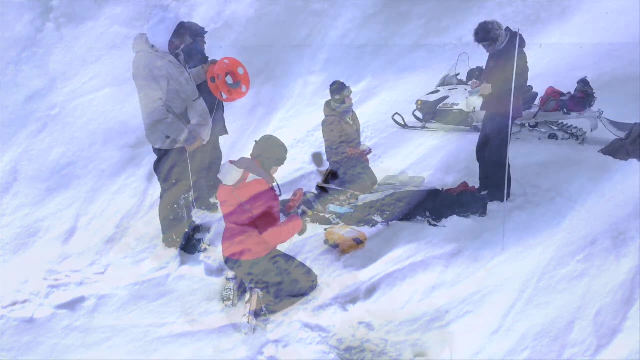 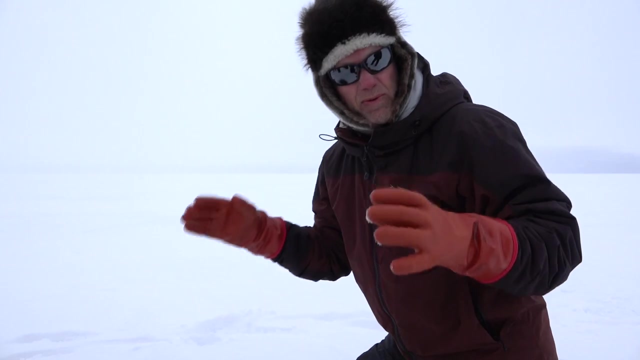 rough pressure ridges or areas with snow drifts that would be deep enough to allow them to construct a lair for having their pups. Our team partners with the National Oceanic and Atmospheric Administration. Peter Boving, a NOAA seal researcher, was able to join the team on a. 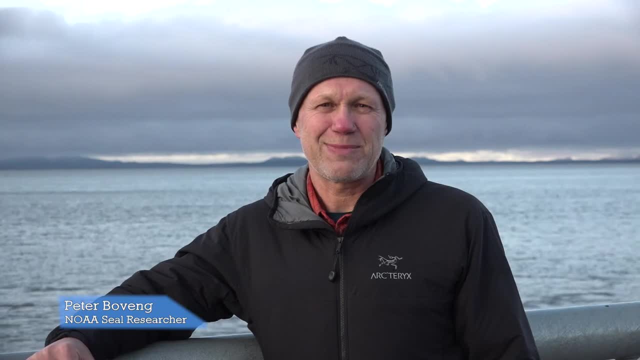 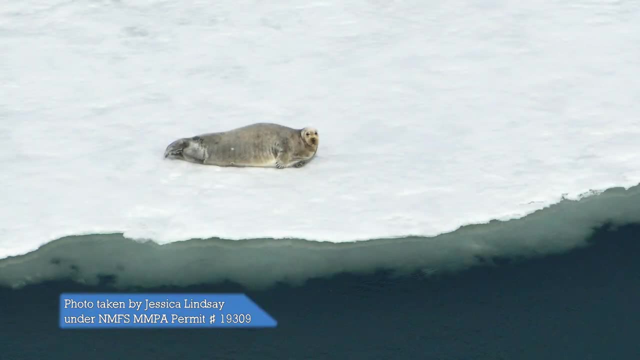 couple trips to Kotzebue. Our interest in participating is bearded and ringed seals. The species are not as well documented scientifically as many of the other seal species in the world. They're challenging to study, They're out in the ice, They're hard to get. 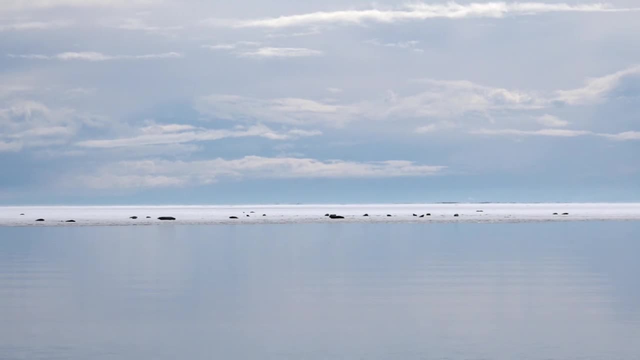 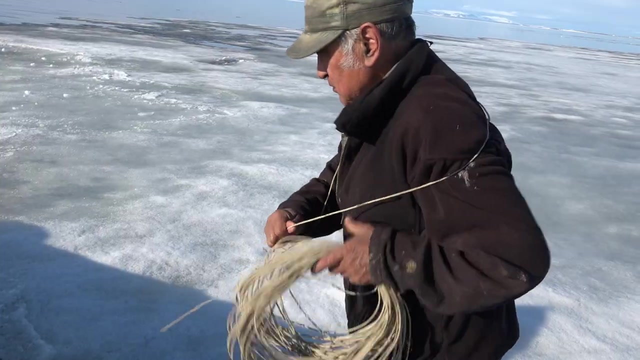 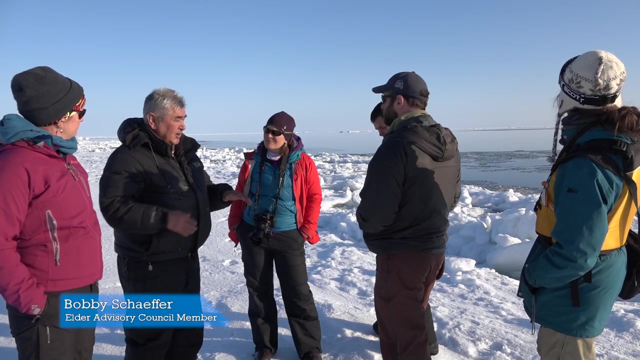 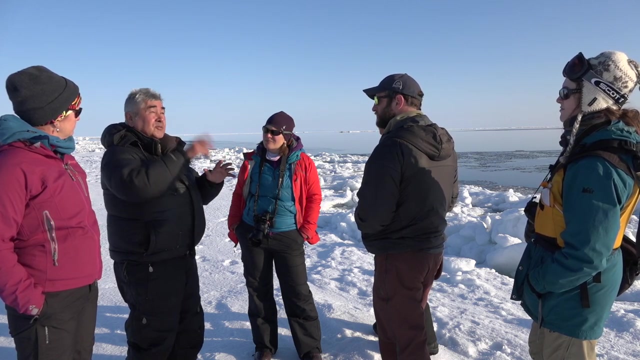 to. It's expensive. We're interested in learning about their vulnerability to changes in a warming Arctic. The elder advisory council members are pivotal to understanding changes in seal habitat. They usually like to go to ice piles because ice piles provide shelter and also they can breathe and it's safe for them. They're from. 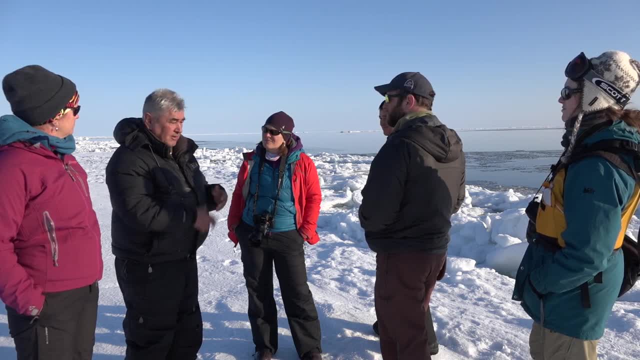 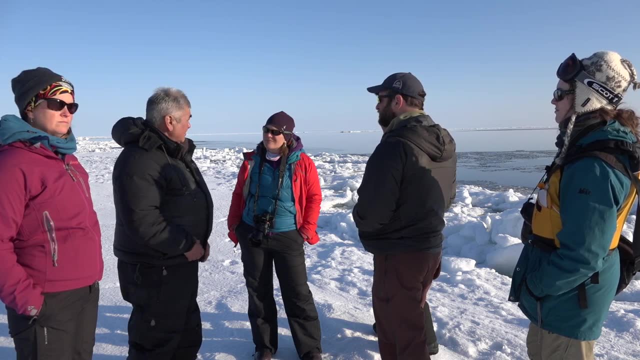 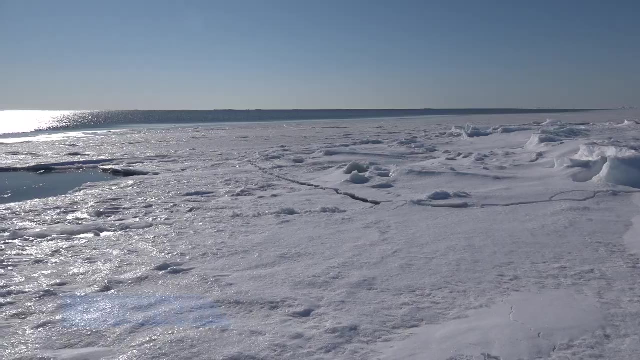 the predators. so the seal pups can grow until they get ready to get old enough to go on their own. But with all this lack of ice, I don't know where they're doing it. I think they found a way. One of the biggest changes that we notice is that the water is much warmer. And, as winters have no ice, the sun warms up the water so much earlier. This will be our fourth year that our ocean has not froze, And the only place that it froze was along the shallow islands that we have near Kotzebue. 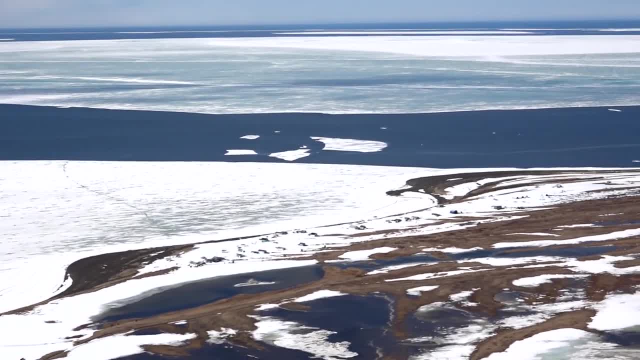 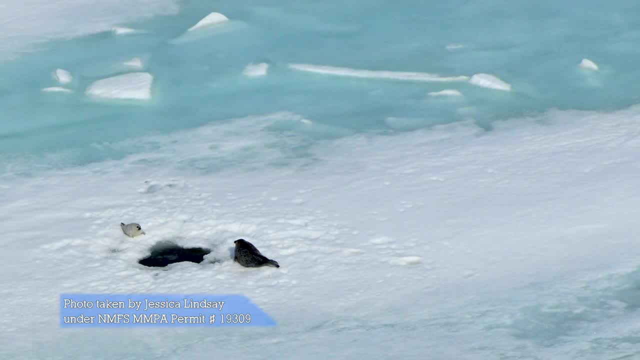 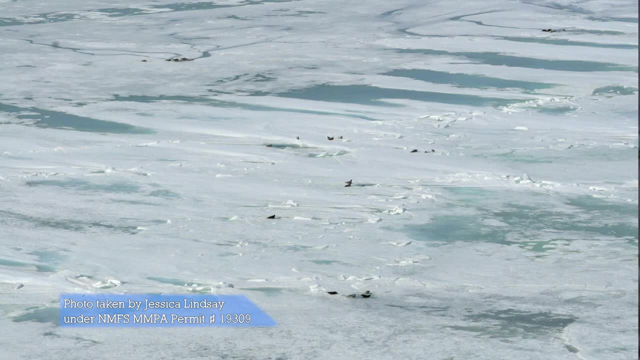 And it presents a lot of problems for all the animals, including the humans. What happens is that the seals have to have their young closer to shore because they've got no ice to go to, except for the Landfast ice, which is four or five miles out to eight miles out and some places only a mile and a half out. 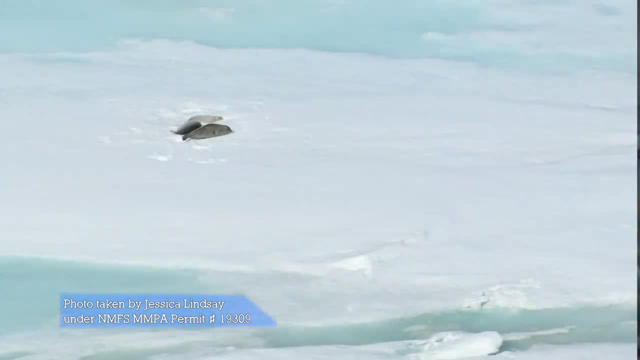 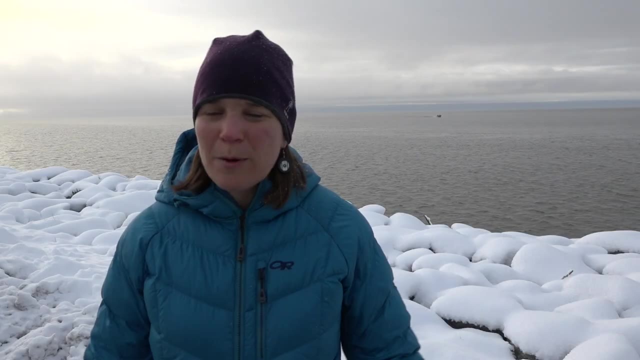 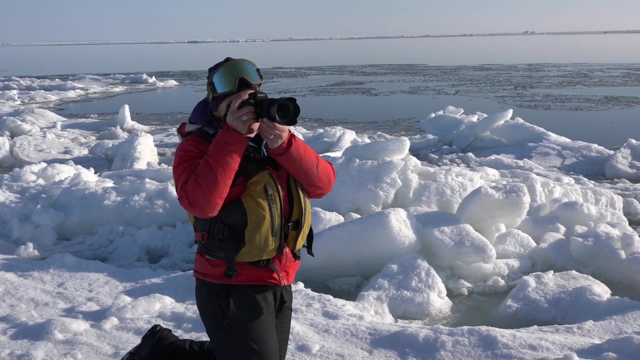 And so they have really no places to make their dens now, because we don't have any big piles of ice like we used to have. There's no question in my mind whether climate change is real. Big things happen. One thing that I always think about is sea ice loss. 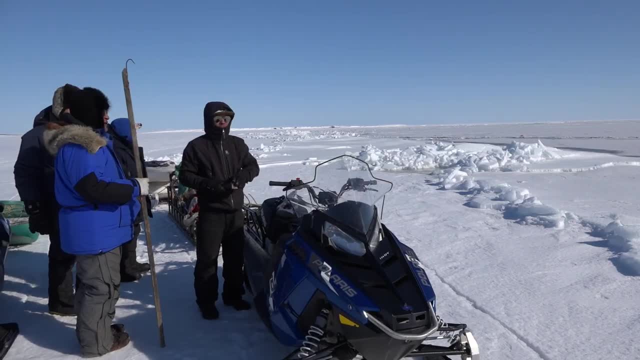 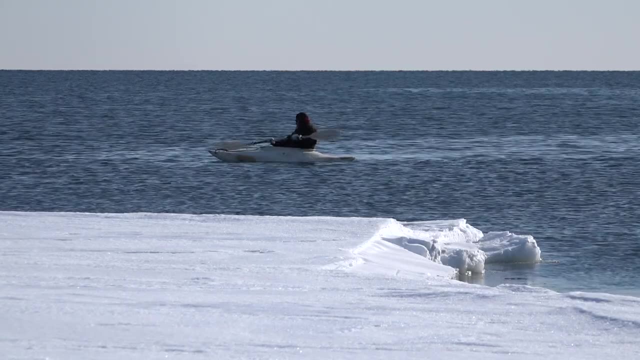 Arctic marine mammals that are ice-associated. How that affects the people that rely on those animals and those species as well. Are there changes in their accessibility and their availability? We've had to modify our way of hunting and we've also had to become very, very careful. 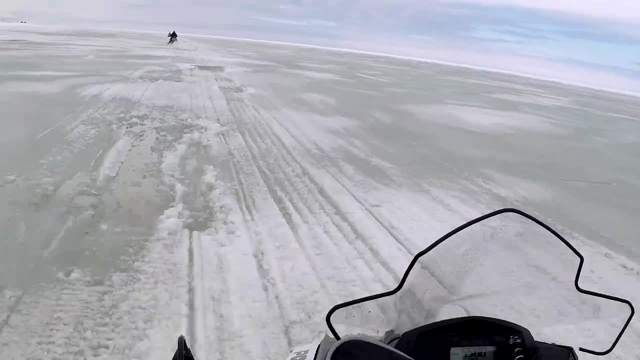 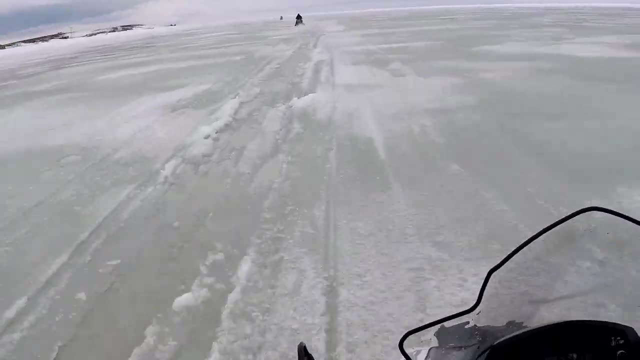 The last two years I have not hunted in the spring because it's so different that I don't want to lose my life Because you can't read the ice. It's not as well as we used to. The way of reading the ice is no longer valid. 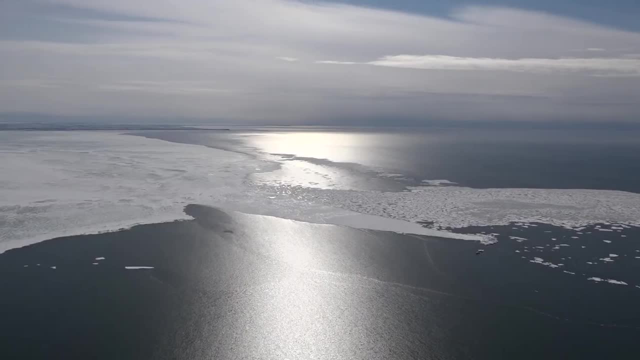 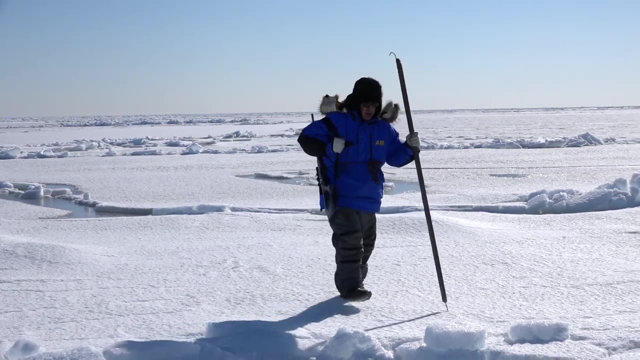 It's changed so much, And our springs and our falls are becoming longer and longer, whereas our winter is shorter and shorter. At one point in time, we used to have nine months of winter. Now we think we have about six months of winter or maybe less. 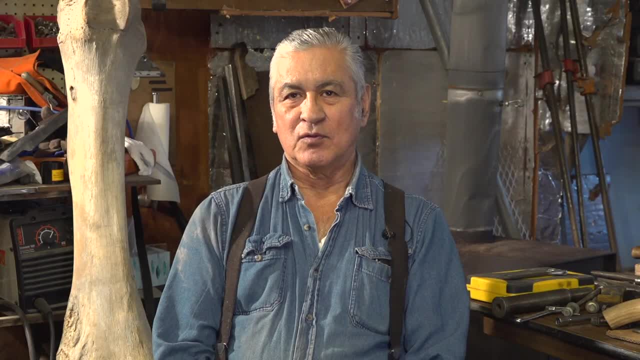 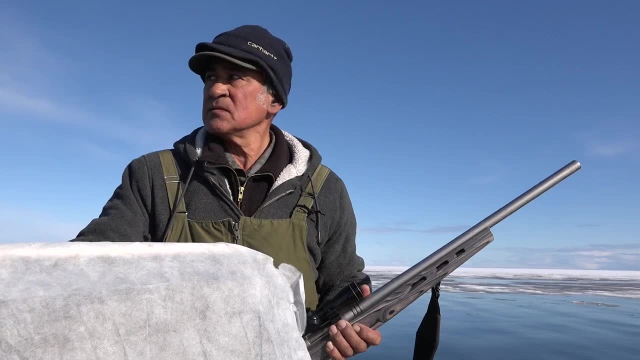 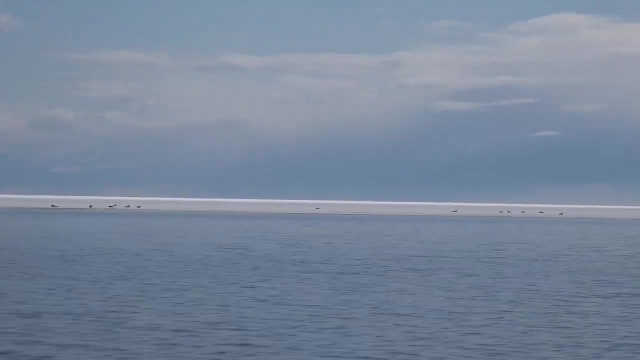 It limits you as to what you can do when you're looking for food. So much of our way of life is not only physical, in terms of getting out to the country to get the food, but it's also very spiritual to a lot of our people. 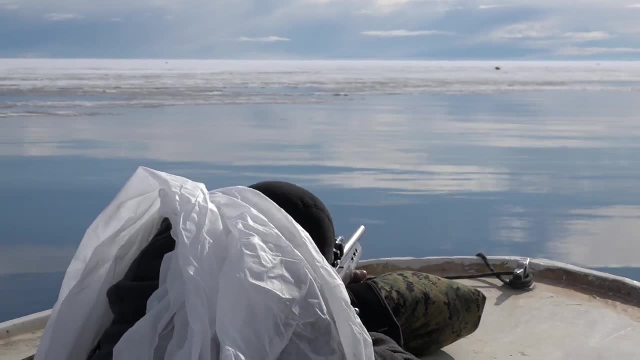 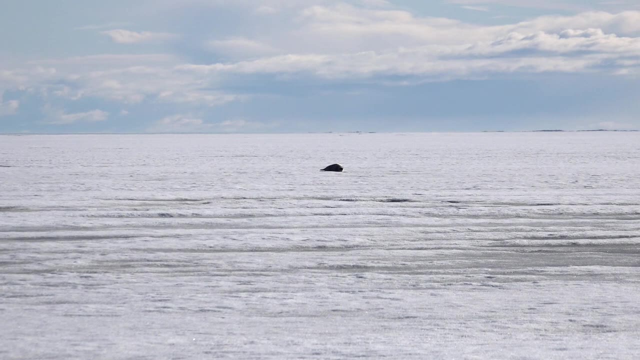 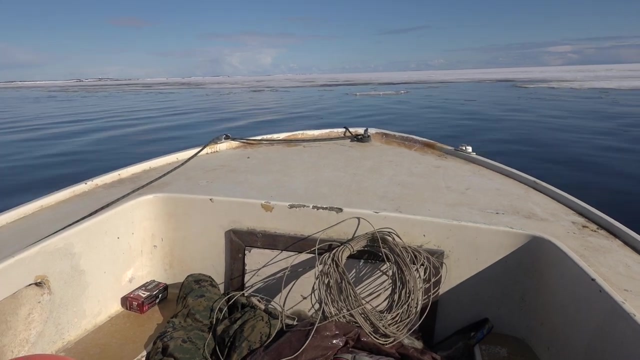 We've done this so many years and there's certain ways to do things that indicate how spiritual it is. Even something as simple as hunting for elders is spiritual, In that when you bring food to the elders, they tell you: thank you.